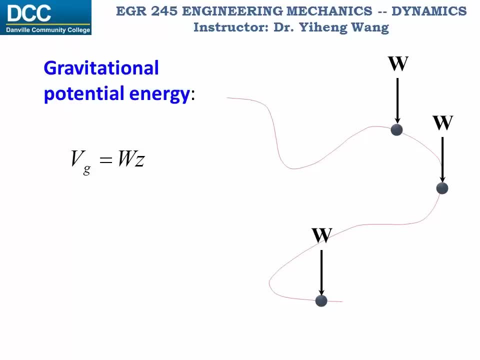 Potential energy is normally denoted by the value of the potential energy. Potential energy is normally denoted by the value of the potential energy And the gravitational potential energy vg, which is the potential energy associated with the weight of an object, equals to its weight, w multiplied by its vertical location, z. 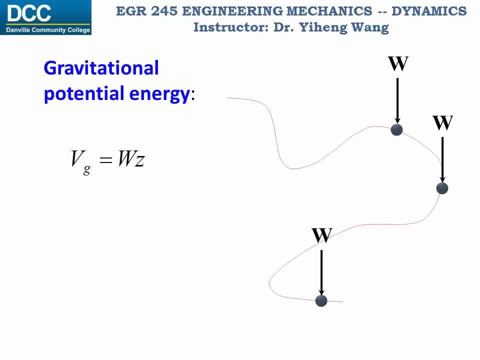 And of course its vertical location can be represented by other letters, depending on what coordinate system you choose. So to calculate the gravitational potential energy, we first need to draw a datum where the vertical location z is zero. So to calculate the gravitational potential energy, we first need to draw a datum where the vertical location z is zero. 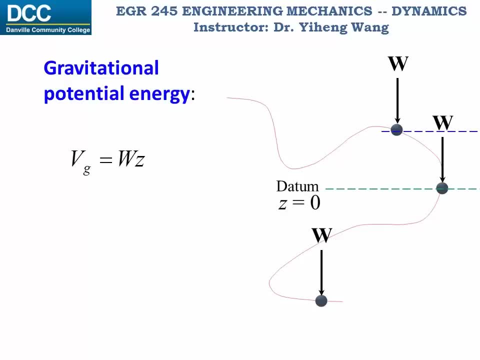 Therefore, for any location above this datum, z is positive and the gravitational potential energy is positive. For any location below this datum, z is negative and the gravitational potential energy is also negative. As you will quickly notice, the value of this potential energy will change if you change your datum. 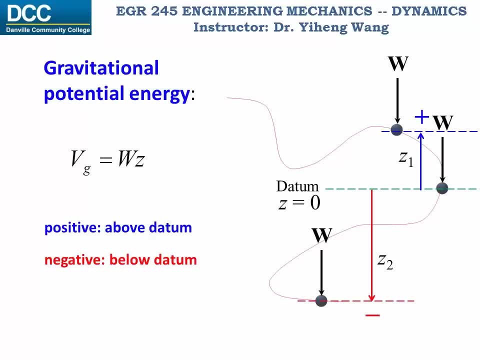 That is correct, but, as I said, the absolute value of the potential energy is not of value. It's not of interest. What's more important is the difference of the potential energy due to the change of the particle's location, And through a quick analysis you will find out that. 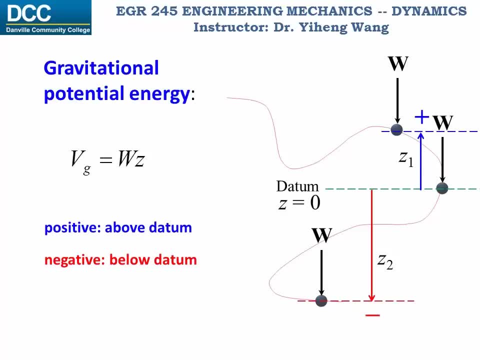 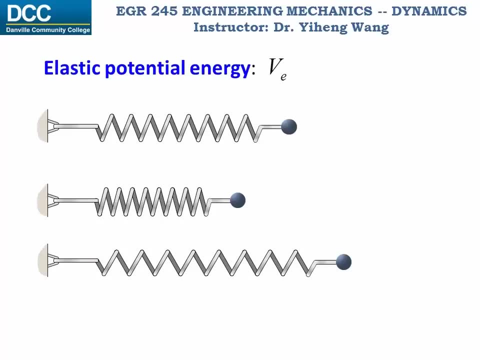 no matter how you choose the datum to be, the difference in the potential energy will stay the same for the state change for the particle. The elastic potential energy Ve is defined to describe the ability of a spring force to do work to an object that is attached to the spring. 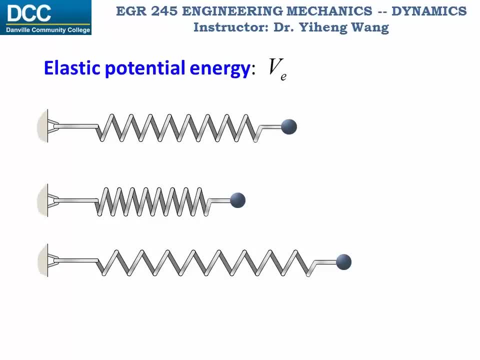 Unlike the gravitational potential energy, the datum for the elastic potential energy is not randomly chosen. It is always chosen to be the position when the spring is unstretched. Therefore, when the spring is compressed, the displacement is negative. When the spring is stretched, the displacement is positive. 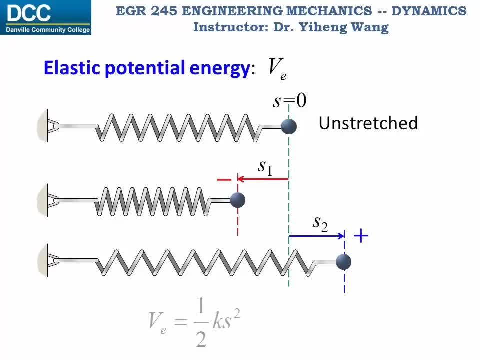 However, the potential energy associated with the spring force is always calculated as one-half k, which is the spring constant times s to the second power. Therefore, it is always non-negative. This is because spring would always try to restore its original shape and length. 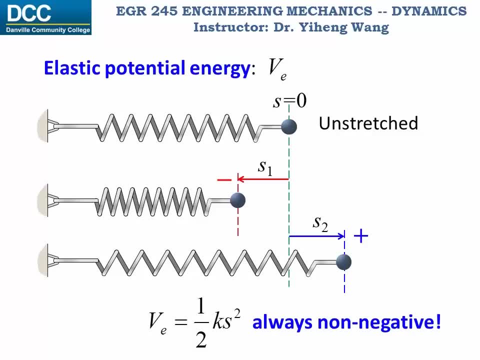 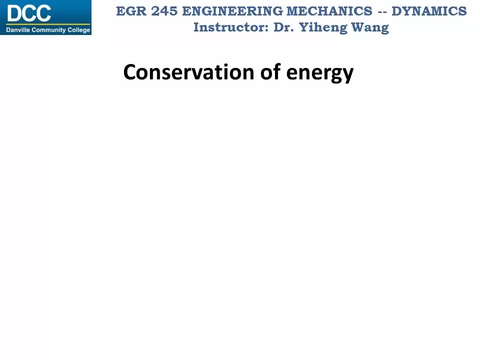 Therefore, no matter if it's compressed or stretched, it will always do work to the particle in order to return to its original, unstretched location. Therefore, with the definition of potential energy, the principle of work and energy that we learned earlier can now be rewritten into the conservation of energy. 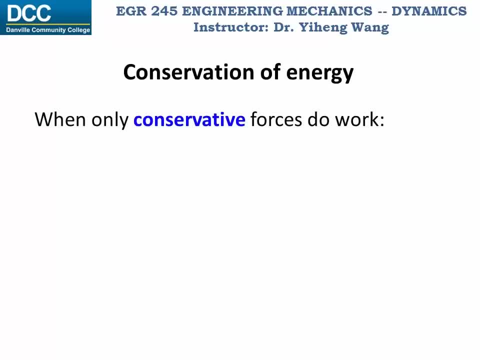 which only applies to the situation when all the forces doing work are conservative forces. In other words, if non-conservative forces, such as frictional force, is doing work, you cannot apply the conservation of energy. The conservation of energy written in the equation is: 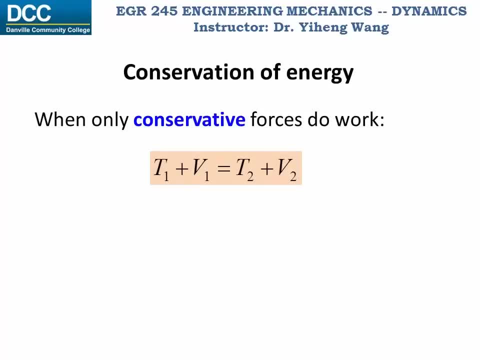 T1 plus V1, the total energy at state one for the particle equals to T2 plus V2, the total energy at state two, T1 again, is the kinetic energy, one-half times the mass, times the speed, to the second power. 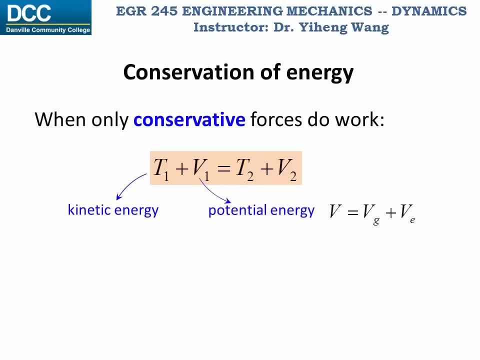 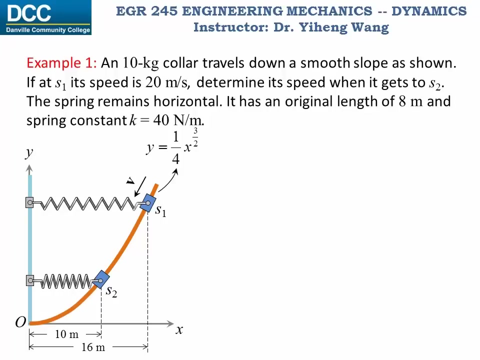 and V. here is the potential energy. that includes generally the gravitational potential energy and elastic potential energy, And the conservation of energy can also be applied to a system of particles, as long as all the external forces doing work to this system are all conservative forces. Let's look at this example. 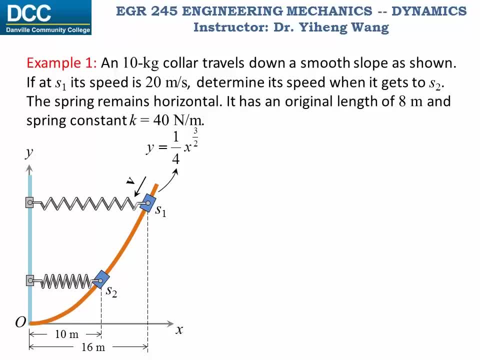 We have a 10 kilogram collar that is connected to a spring. It travels down a smooth slope. If initially it has a speed of 20 m per second, we need to determine its speed when it gets to the second state For this problem: since the slope is smooth, we can neglect the friction. 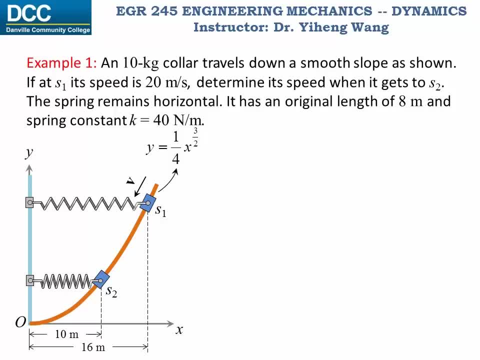 therefore, the only forces doing work to this collar during this process are its weight, as well as the spring force, and both of these two forces are conservative forces. Therefore, instead of applying the principle of work and energy, we can now apply the conservation of energy to solve this problem. 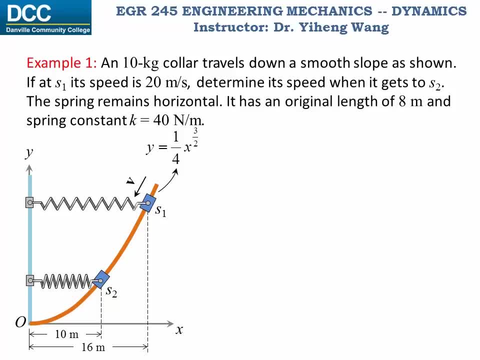 So let's first calculate the total energy of the collar at state one which includes its kinetic energy and its weight And its total potential energy. For its kinetic energy it is evaluated as one-half times its mass, times its speed to the second power, which equals to 2,000 joule. 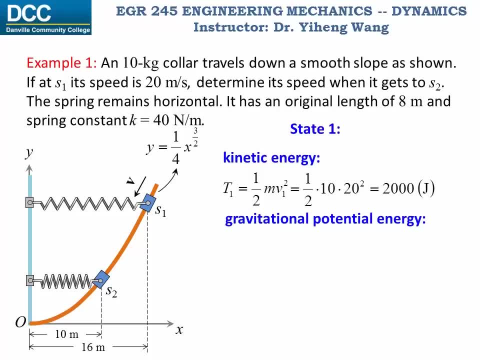 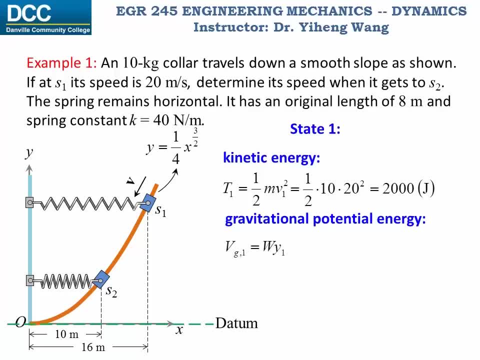 to be along the x-axis. Therefore, its gravitational potential energy equals to its weight times, simply y1, its y coordinate, which can be determined from the equation of the slope, and therefore its gravitational potential energy is determined to be 1,569.6 joule. 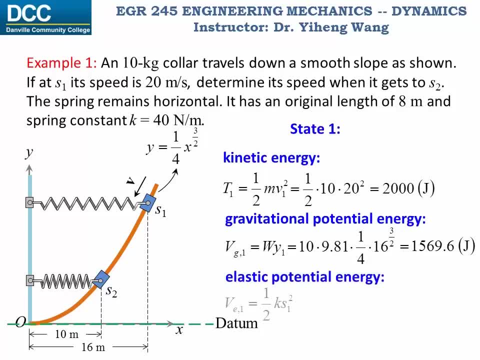 For its elastic potential energy. we know that it is calculated as one-half k s squared. k is the spring constant, s is the displacement always compared to the unstretched length of this spring. Therefore, it is determined to be 16 minus 8 meters. 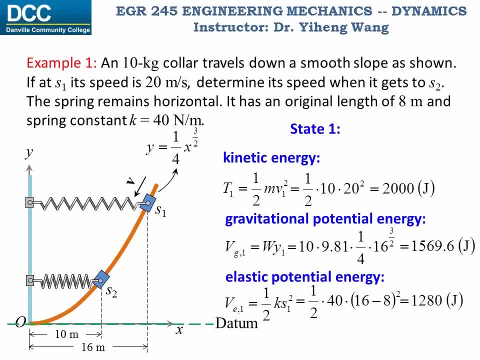 and from here we can calculate: the elastic potential energy is 1,280 joule For the total energy of the color at state two. again, it includes its kinetic energy, which equals to one-half times its mass times, v2 squared and v2. here is the unknown that we need to solve for in this problem. 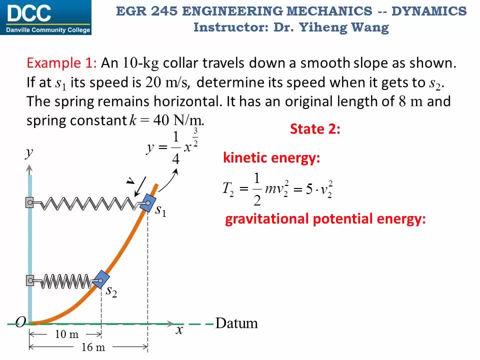 Also the gravitational potential energy. that must be calculated based on the same datum that we used earlier to be w times, y two, and y two is again simply the y coordinate that can be calculated based on the equation of the slope and also the elastic potential energy. 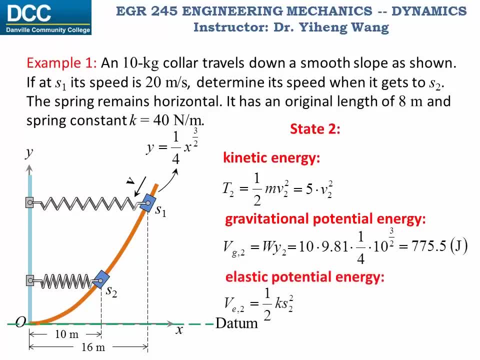 and y two is again simply the y coordinate that can be calculated based on the equation of the slope and also the elastic potential energy, again calculated from the equation, and S2, here again is the displacement as calculated from the unstretched original length of the spring.